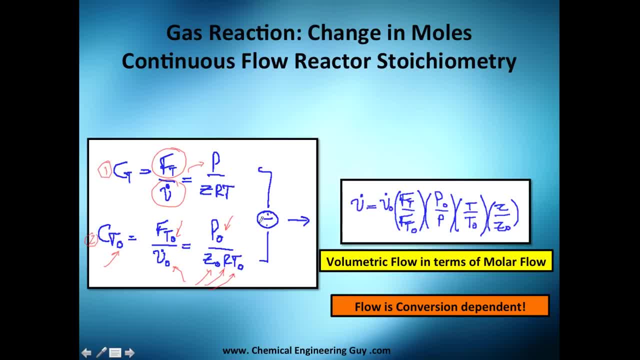 changes. So you got this equation one and you got this equation two. Please divide it and you will find out that actually, just divide this here and this here And look out for V0, no for V. So you take away V0. 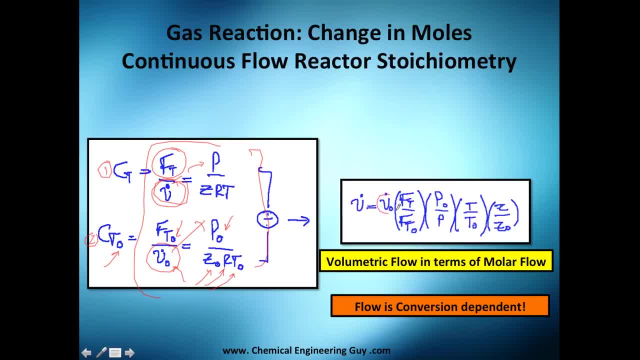 You get this value: Volume equals initial volume times this factor change, which is huge You got. how do they change the flows? How do pressure changes? How do temperature changes And how does this C compressibility factor changes? So one thing: here we have a volumetric flow in. 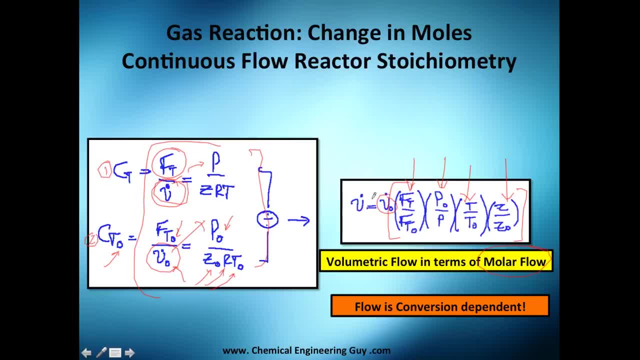 terms of molar flow. Of course volume depends on the flow, But important thing to mark or to tell you is that the flow is conversion dependent. So flow of any subject is function of the conversion of A. As you get more conversion you're going to get different flows. 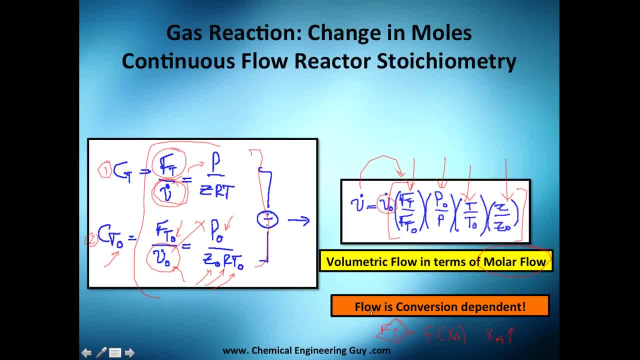 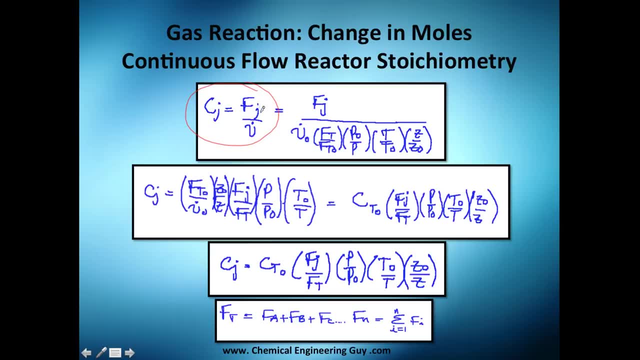 So let's try to force the conversion into this equation. So, at any moment, we got concentration of J equals flow of J divided by volumetric flow rate at any time. So we already got one expression for this, which is this huge stuff here. So let's substitute it and we have everything or all. 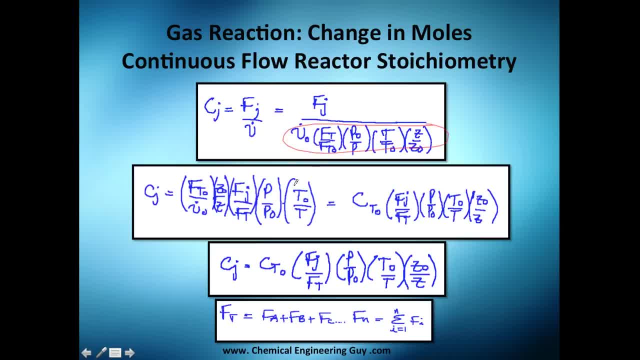 the equation here. Now let me just do some algebra. I'm not adding or subtracting stuff, I'm just arranging. I got this Ft0 divided by V0, the C's stay here, the flows, the pressures, the temperatures, And, if you remember, this is the definition of concentration or initial. 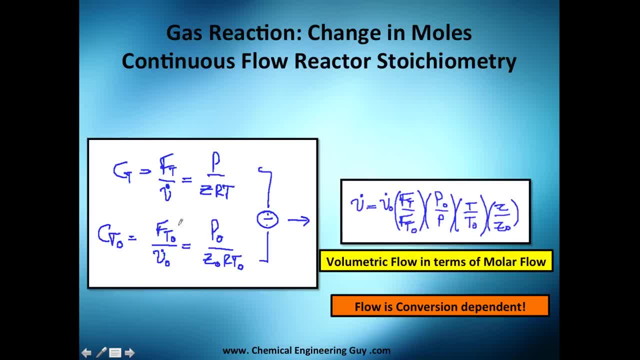 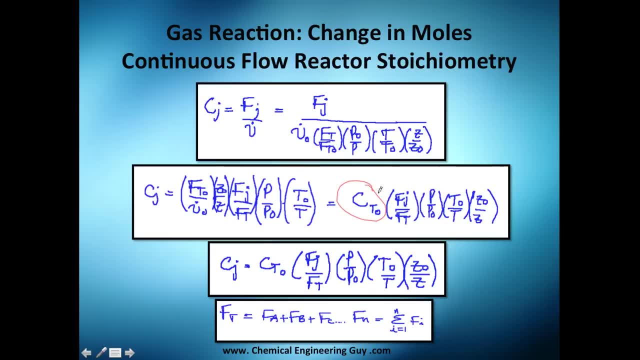 concentration. Let me go back So it appears again. Good, Now we got this. total concentration times the effect. Now what else can we do? Okay, This is valid for anything, For A, B, C, D, Whatever. The only thing it changed is this. 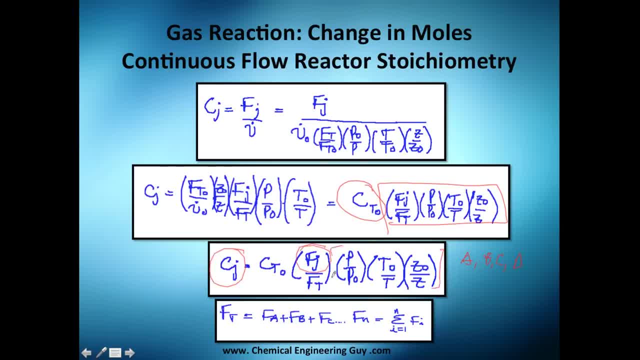 concentration and this flow. Everything is fixed. For example, the pressure is the same for any species. Temperature is also the same for any species. The compressibility factor is also the same. The initial concentration is a. the total flow, of course, is the same. The only thing you got different is the. 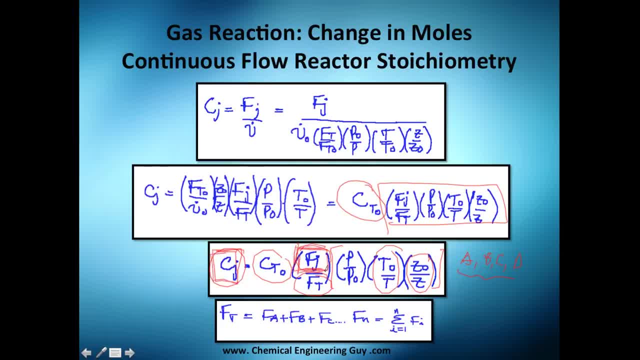 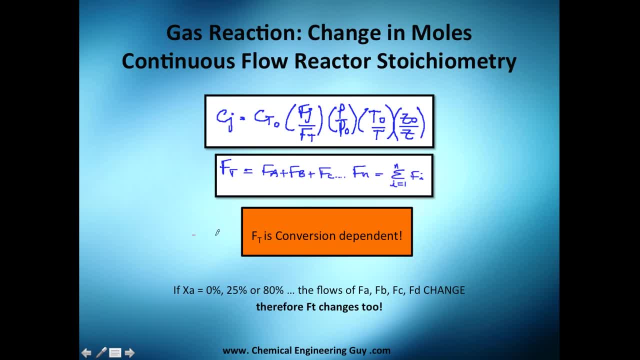 concentration, which is based in this variable flow. Okay, we got this. One thing I want to tell you is that f of t, or the total flow, of course depends on the conversion. Why? Because if you know that f of a depends on x of a, f of b depends on 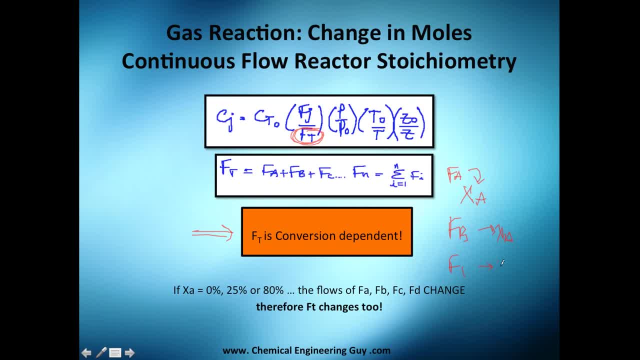 x of a, F of c depends on x of a. So as x of a increases, f of a decreases, f of b decreases, f of c increases, f of b increases. So what I'm telling you is, as the conversion of a goes to 100, you're going to increase products and you're 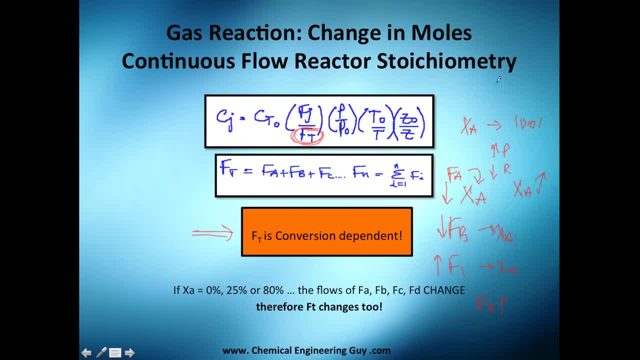 going to decrease reactants. So, of course, if I have x of a at 20%, I'm going to have different value of flow or the total flow, as if I were to compare X of a, let's say 80%. Okay, of course, at 80% I'm going to. 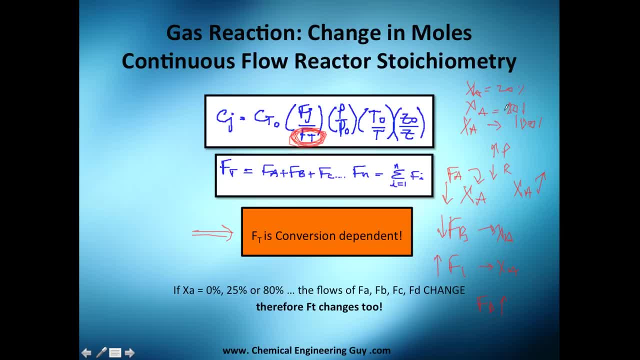 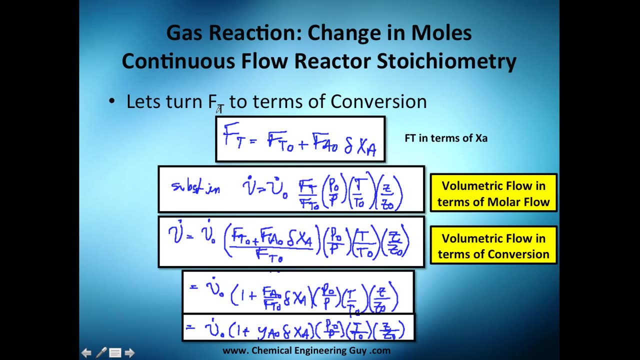 Have more products and those products may be moving the total amount of flow right here. So just keep in mind that f of t changes with conversion. Now let's turn the flow, the total flow, to terms of conversion. That's what we want. We don't want to have f of t. 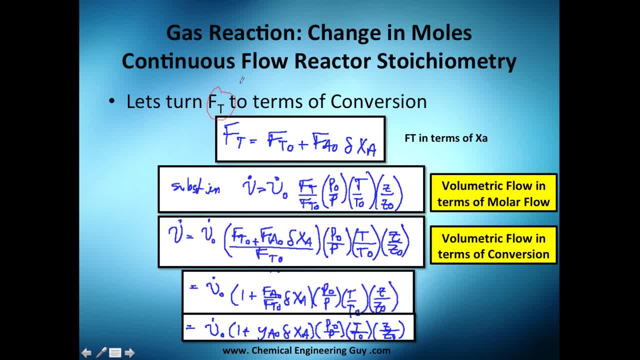 It will be cool if you can change everything to conversion. So how do we get that? we can do it and hopefully you remember where do we got this? if not, go back to the patch and To the CST or the continuous tank reactors and check out where do we got this definition? 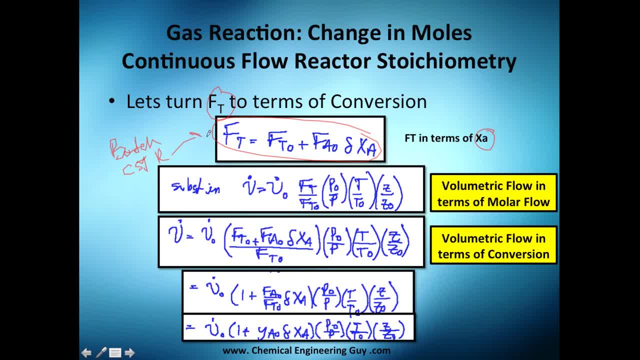 So let's go back to the CST or the continuous tank reactors and check out: where do we got this definition? By definition, the total amount of flow is given by the initial amount of flow plus the change in volume, which is here, or the change in moles, and 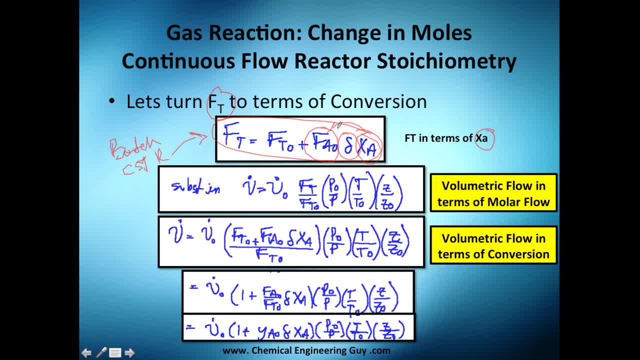 This guy times. this guy will give you the change in conversion. Now, How do we Flow in terms of molar flow? okay, Let's substitute this new equation. Let me take away that This new equation will go And we're going to substitute it here. 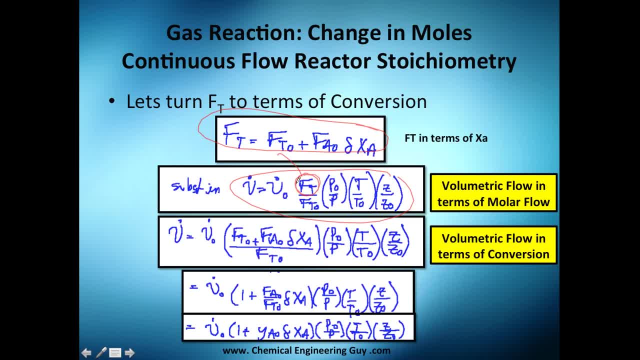 But we're exactly in this part right here. The good thing is that everything else is constant. case T is a constant T series, a constant C and C series, constant P 0 P Constant and volumetric flow rate is also constant. The only thing that is not constant is this flow or total flow at any moment. 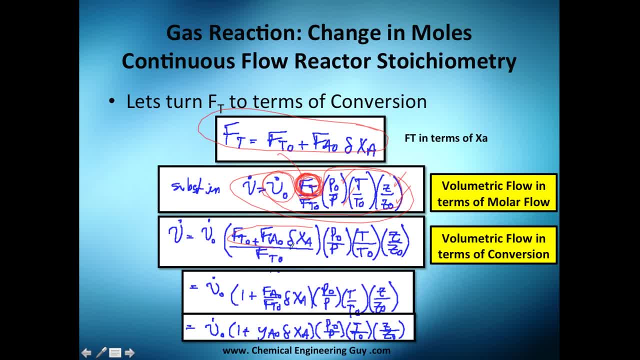 so yeah, let's suppose we just substitute that here and You can see this is 1 to the left, and we get this, Which is actually the mole fraction, and you get this: Delta times X of a. So let's change this to Y of a and let's continue. 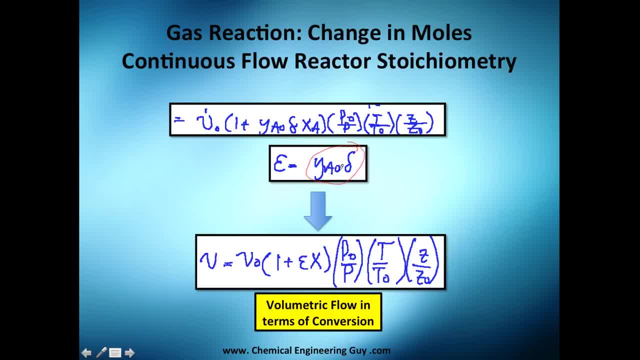 Remember that by definition Epsilon is the mole fraction of a at the beginning times the change in moles. So this here is epsilon. I'm just going to substitute epsilon, and Probably you are more familiar with- 1 plus epsilon X, then pressure, Then temperature, then C. 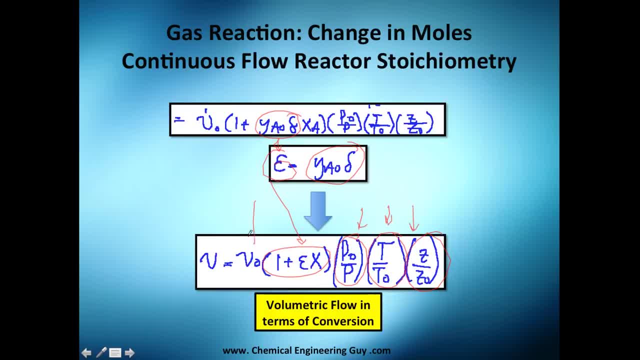 Factors. these are factors. These are constant. The initial volumetric flow rate is also constant. So, as you can see, now we have volumetric flow In terms of conversion, because this is constant. This is constant. Epsilon is also constant. The only thing that it's not constant is X, and that's awesome, because now 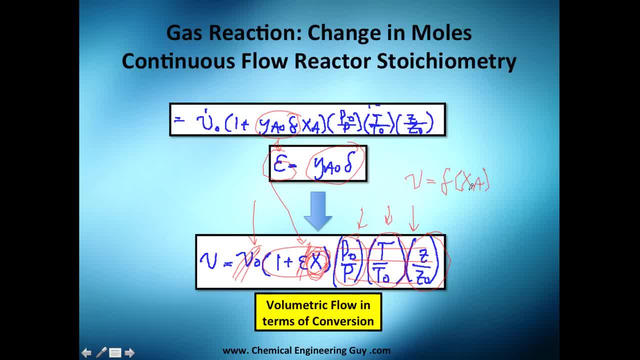 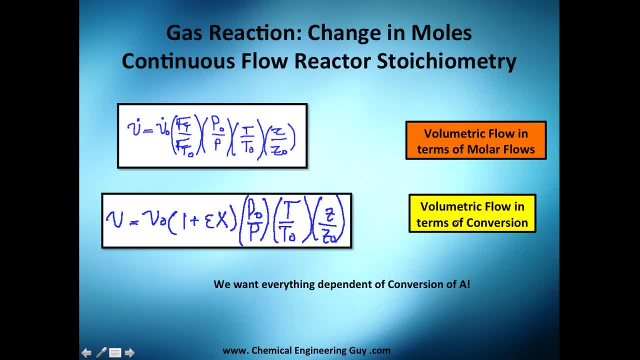 We have a function of conversion. So we got this before in terms of molar flow, but we don't want that, we want in terms of conversion. So look how we change this thing to this thing here. Everything else stays the same here. Okay, Good. 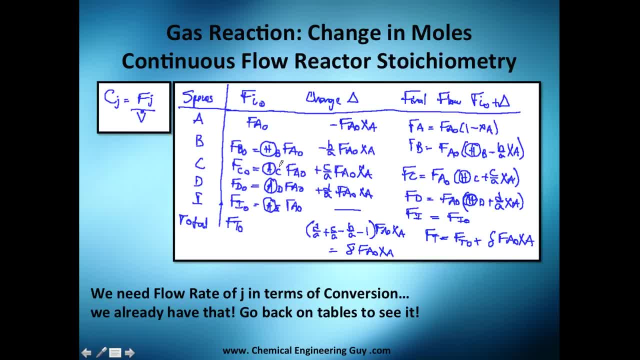 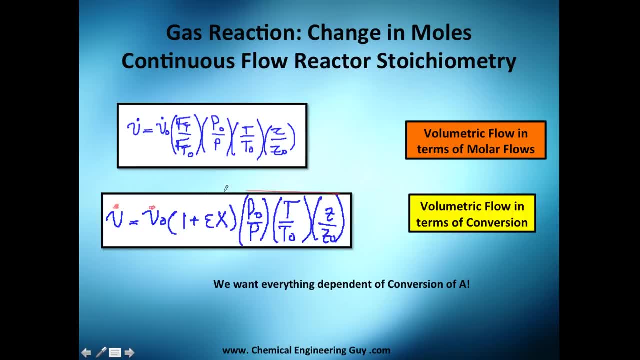 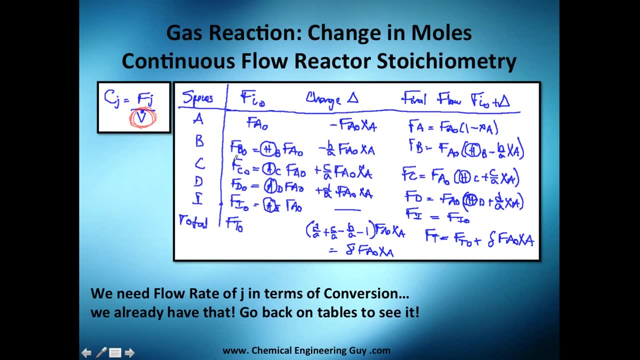 Now Things are going more tricky. We're going to substitute that volumetric flow rate, So you have it here, so we You need to have this here. We're going to substitute all this huge stuff in here in this conversion. Okay, So, if you remember this table, please, 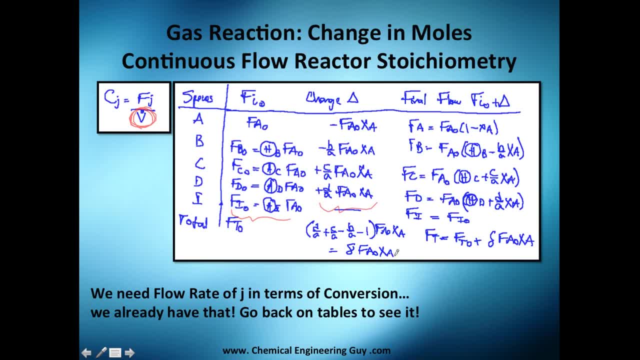 recall this table and you have this and you have this. and The thing here, guys, is we need flow rate of J in terms of conversion. What's that? We need This here, this here, this here and this here in terms of conversion. So how do we do that? Let's change everything to. 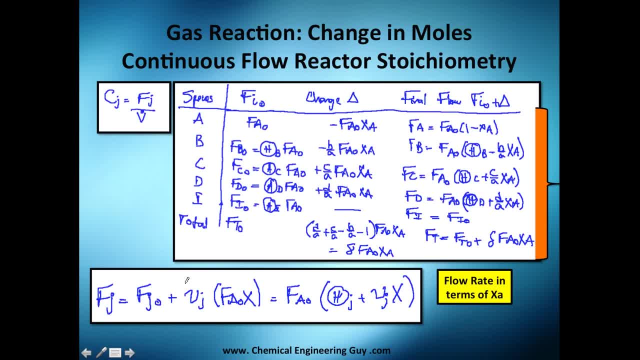 conversion. How do we do that? As we've done before, you've got this initial flow rate. This is the coefficient. Let's say B divided by A or C divided by A or D divided by A. We're going to see that for a reactant it's positive, for products it's positive. 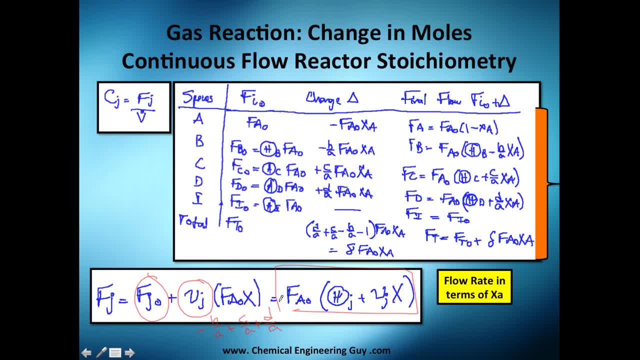 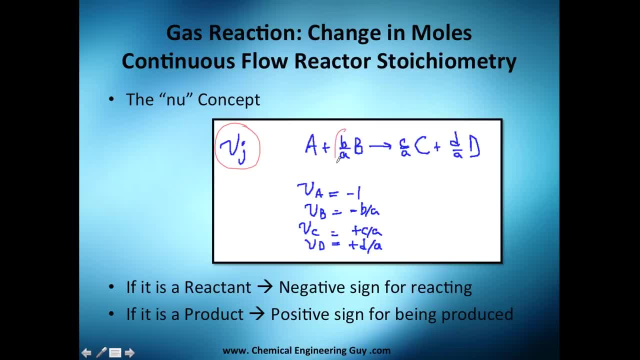 Then we get this here. Let me go here. Oh yeah, that was what I was explaining you. What is this new value? Well, this value here, this value here, this value here and this value here, of course, For A, it's always minus 1, for B, it's always minus B divided. 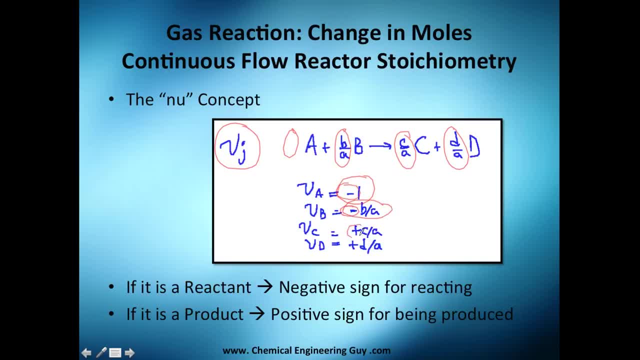 by A, because it's a reactant product and, yes, you got this. The importance of this is that when its reactant is negative- please, guys, don't forget that- and the product is a positive sign. now, once again, let's go back here. 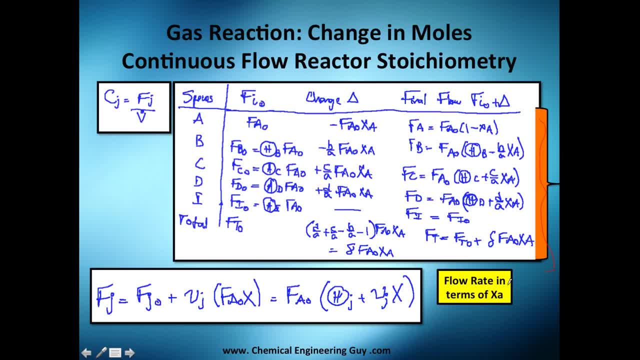 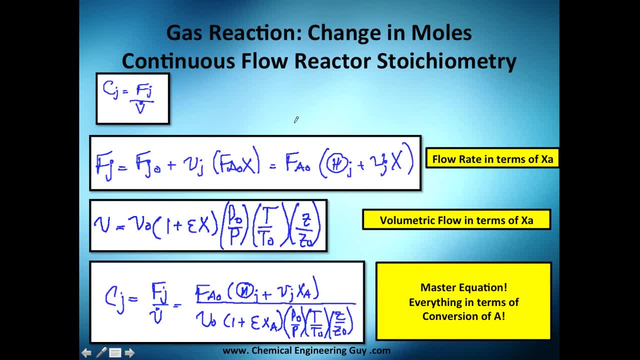 we're going to make our analysis here. we want those flow rates in terms of conversion, so let's continue. we got, we have this equation, okay, it's valid for every species. now we got this in terms of conversion and we want this in terms of conversion. and the thing is we actually have 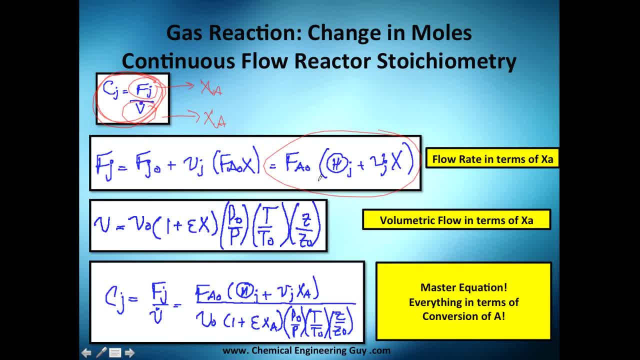 done it recall, we just got this value before and we got this value a little bit before. so everything depends on the x and x, everything else, this value, this value, this value is constant and this value, this value is also constant. so you have two equations that depend on the in x. 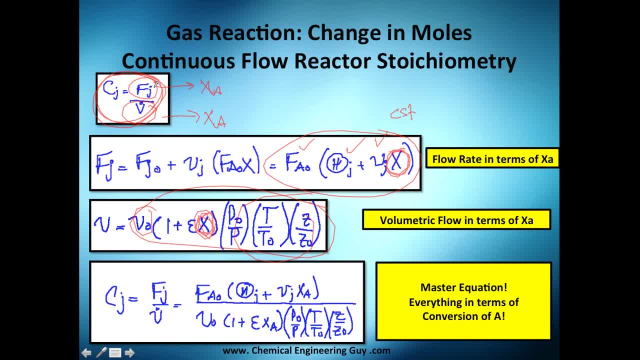 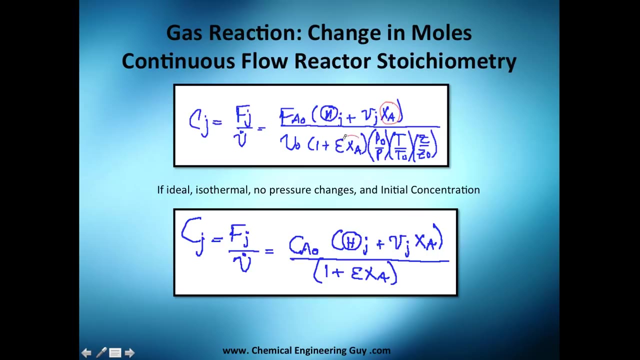 and what means that? that if you divide that equation and that other equation, they will still depend on x. so we got our master equation here. fj is here and the volume is here and, yeah, everything is in terms of xa here, xa, xa and if ideal, isothermal and not pressure. 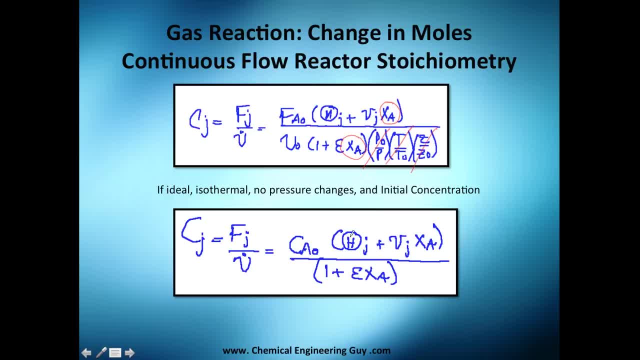 changes, so not pressure changes. isothermal and ideal gas. we will get this equation but done. i think we're going to use always this equation. we're going to use these equations the most. this is just the case in which it's isothermal ideal gas and there's no 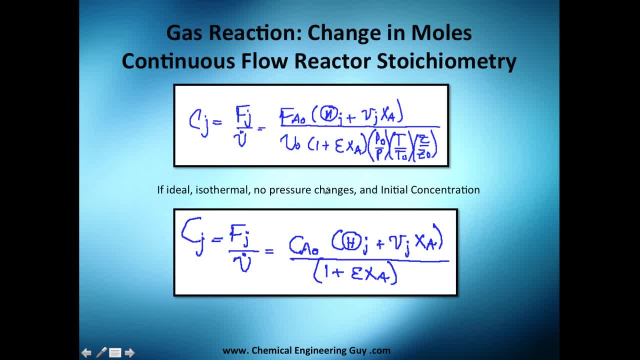 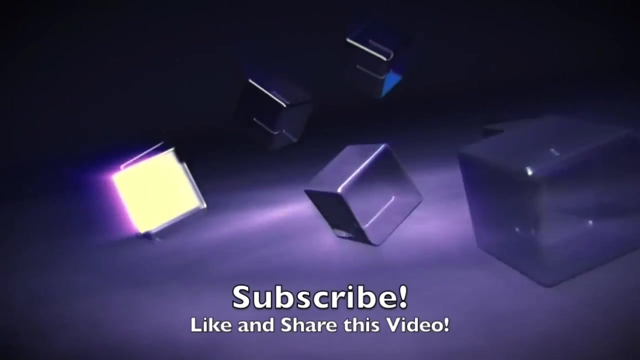 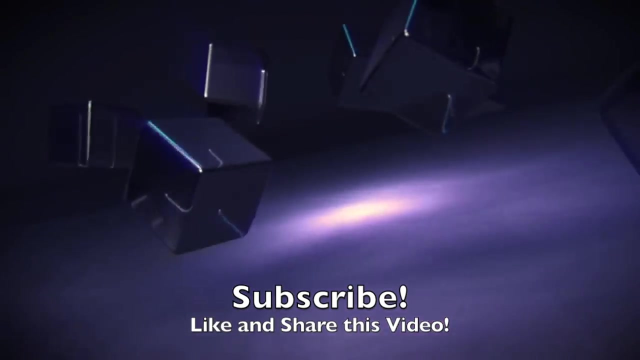 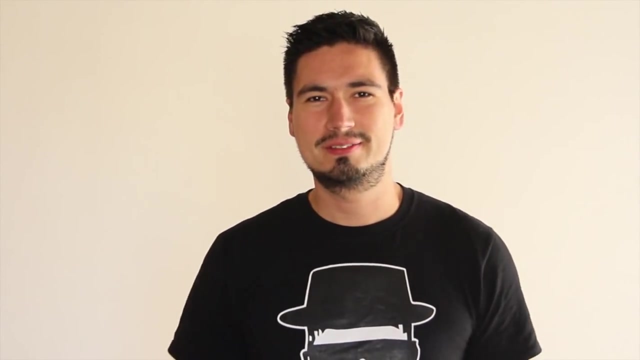 pressure loss. so i know, guys, that you are probably overwhelmed with many equations and many things, but i'm going to make you a summary, a visual summary, so you can get to understand what we done in these four, five videos. so good luck on getting not confused. what's up, guys? it's me chemical engineering guy. so if you like the video, why not push the like? 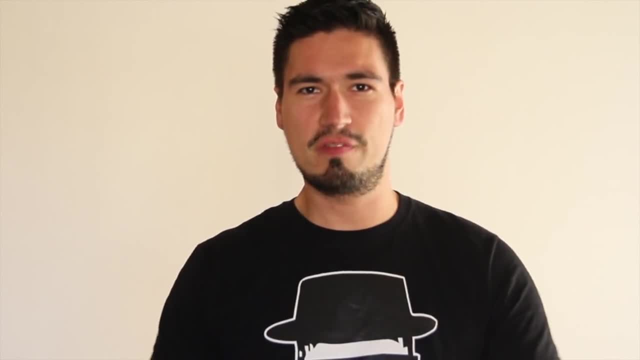 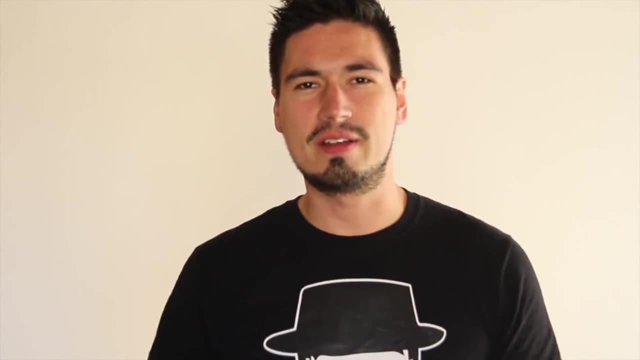 button. it really helps me to know if you're liking the videos or if i should be changing something or i should be adding something, or if i should be adding something or if i should be taking out content. whatever also, sharing is caring. so if you got any kind of friends teachers, 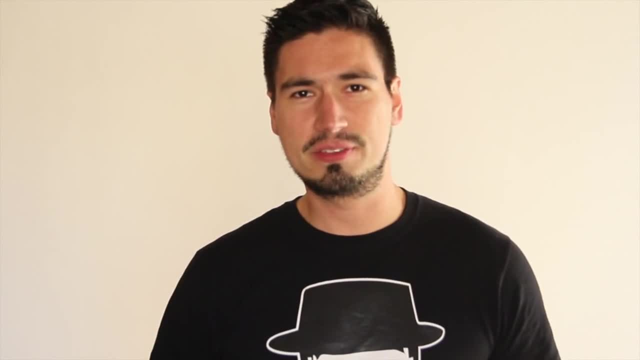 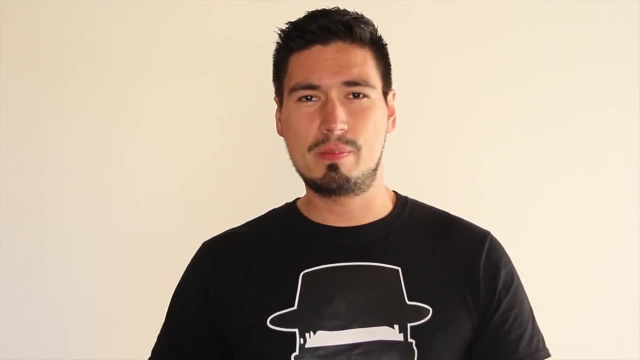 colleagues or whatever kind of person that might be interested in this type of content. why not share it? sharing helps our community to grow faster- in members and in content. if you want to keep track of my activity- videos, uploads, experiments, plays, whatever content i'm getting youtube, be sure. 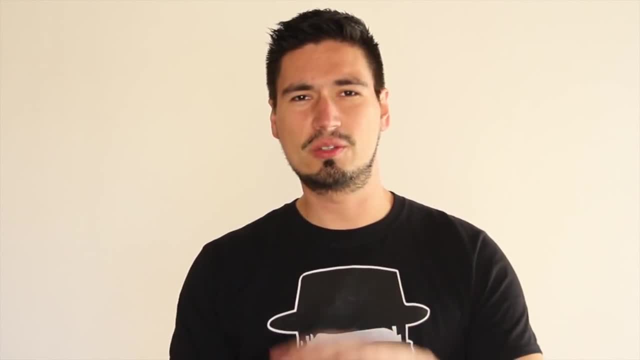 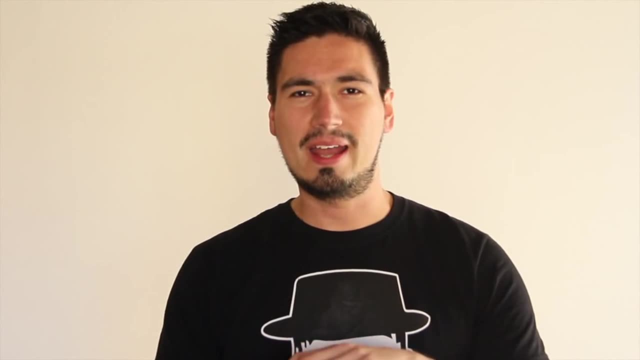 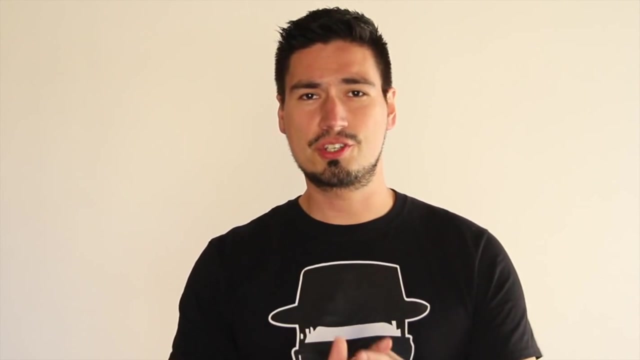 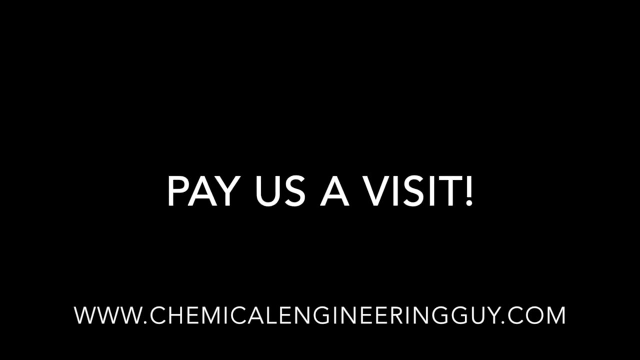 to click the subscribe button. subscribing to the channel is totally free, guys. my dream is to create an online academy of chemical engineering where everyone can access it in the world. imagine a place in which the student, the teacher and the engineer get the best of each other. so thank you, thank you. thank you, guys, for the support and the love.